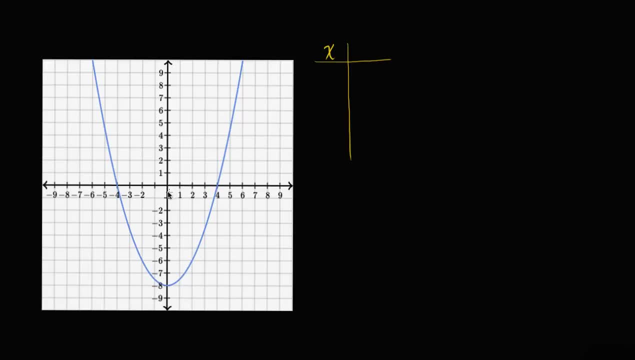 view as something of a function definition. So, if x is equal to 0, as x is equal to 0,, what does this graph tell us? that f of x is going to be? It tells us that f of x is going to be equal to. 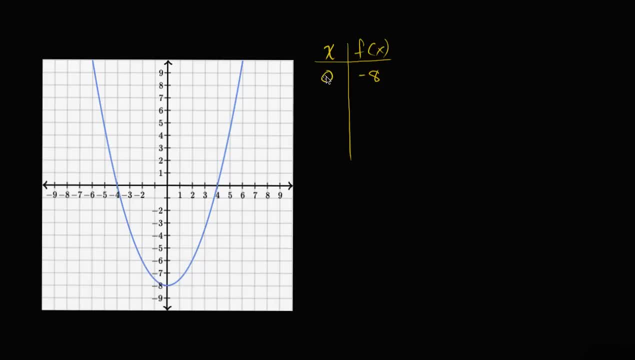 negative 8.. Fair enough, It took 0 as an input and it mapped it to one value, to negative 8.. Now, if x is equal to 2, what does this function map it to? Well, f of x is negative 6.. Well, that's all fine. 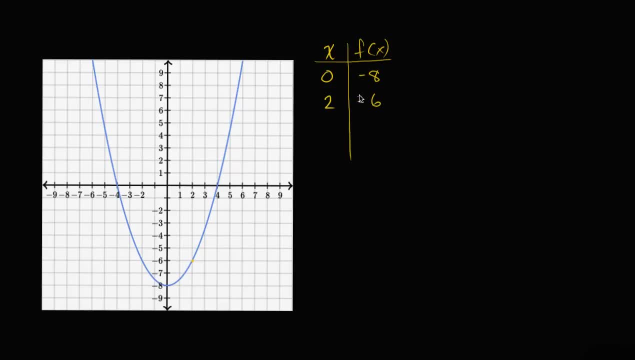 It's just taking this value and it's mapping it to negative 6.. Now, what if x were? what if x were negative 2?? If x were negative 2, it also maps it to negative 6.. Now, this is all okay for a function. 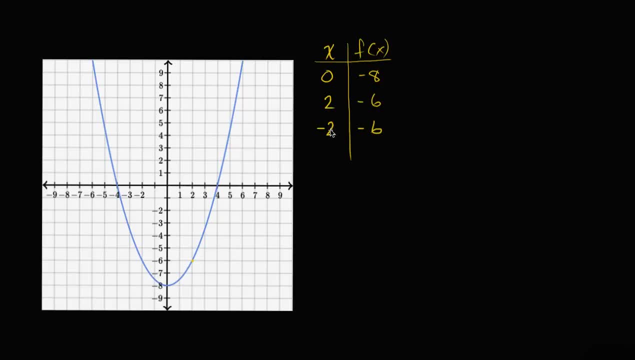 As long as when you give it a value it can spit out- it knows which value to spit out- you have a legitimate function. You could have two inputs map to the same value, just like we had over here Another way to think about this. 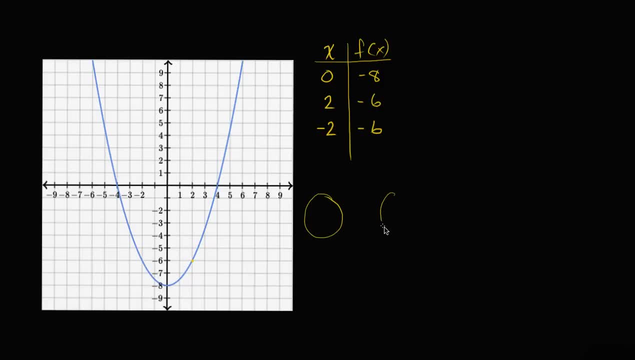 is if you have your domain and then you have your range. So this is the set of all the valid inputs into your function And then the range, and the way we talk about range is really the image. This is a set of all of the valid outputs of your function for 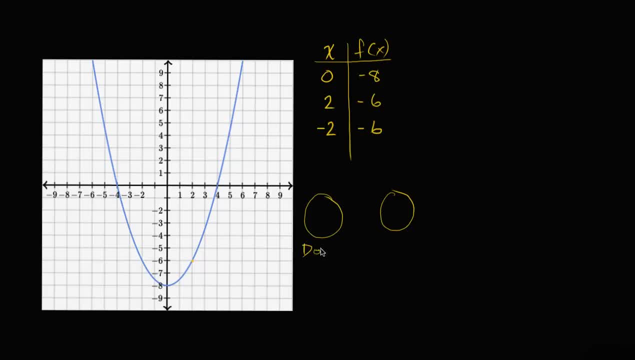 each of all of these valid inputs. So this is your domain domain and this is your range. What we just saw over here is that the 2 maps to negative 6, negative 6, and that the negative 2, negative 2 also maps to negative 6.. 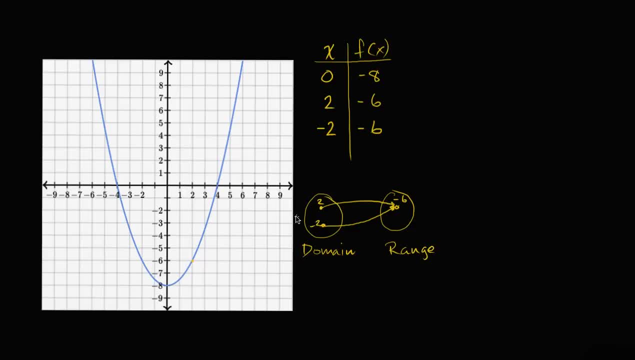 Which, once again, it's completely fine for a function. You would have an issue. This would no longer be a function if 2 could map to two different values, If 2 could map to negative 6, or if 2 could map to negative 6 or say 7.. 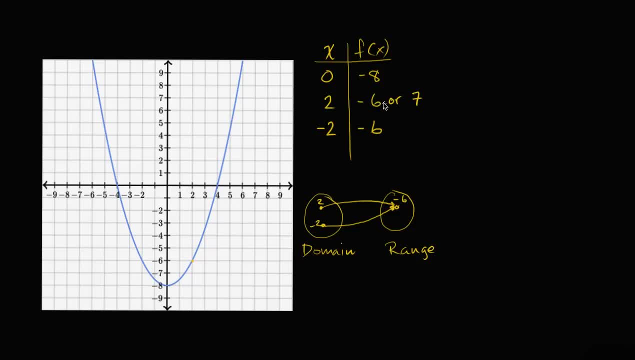 Now, then this is getting weird. Now this is no longer a function where you could get two possible values being outputted for a given input, But that's not what's happening right now. So just what we've drawn over here, this looks like a function. It's completely legitimate. 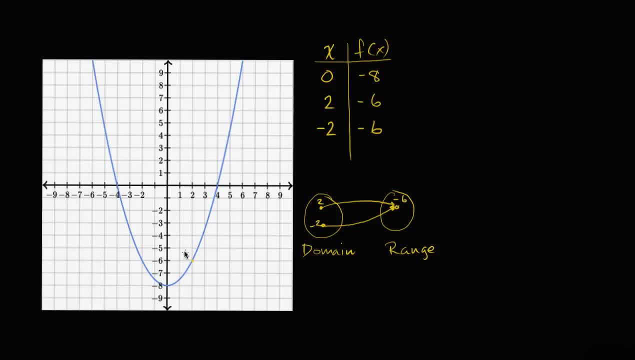 And one of the tests that people make sure that for each input you only have one output is often called the vertical line test, where you take a vertical line and you say, okay, does it intersect the graph of the function? only once, Because that says, well, for each value of x do you only have one possible value of your. 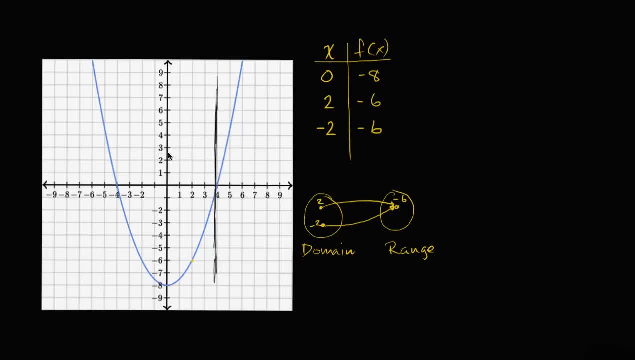 function. One possible value of y is equal to f of x, And so this is clearly a function. Now the next question is: is it invertible? Because in order for a function to be invertible, you should be able to find a function that maps the other way. 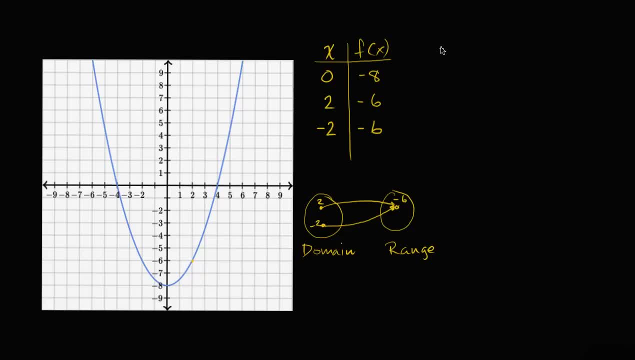 So you should be able to take. you should be able to take a- let's call it a. y equals f of x. You should be able to take one of those and then apply your inverse function to it. Apply your inverse function and get the x that would give you that y. 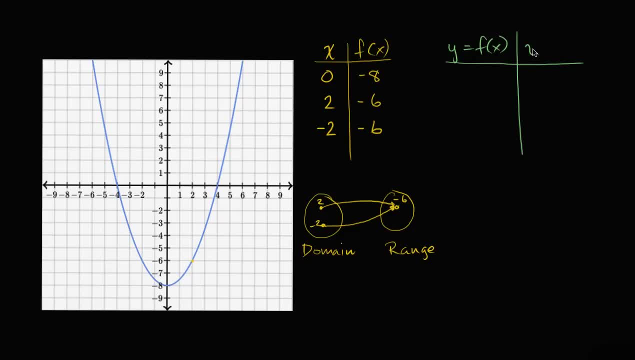 So you should. that should give you, so you should be able to get. x should be the inverse, So it should map the other way. So what am I talking about? Well, if you input a negative 8, if you input a negative 8, well then that should go to a 0. 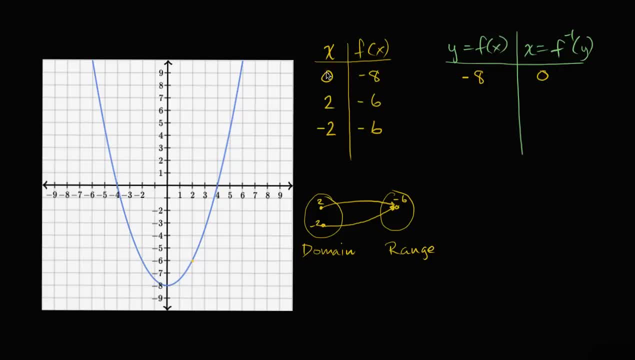 It's going the other way. It's going the other way. The inverse function, instead of mapping from the function, maps from 0 to negative 8,. the inverse function will map from negative 8, will map from negative 8 to 0.. The input into the function that you would have had to get. 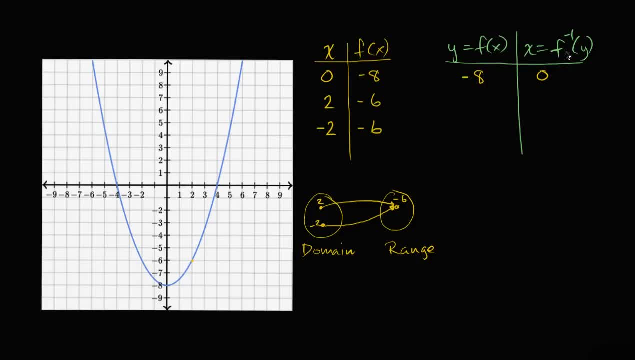 to get to negative 8.. And we call that f inverse. So you could say f inverse of negative 8 should be: f inverse of negative 8 should be 0. I could even write this. I could write this as: f inverse of negative 8 should be equal to 0. 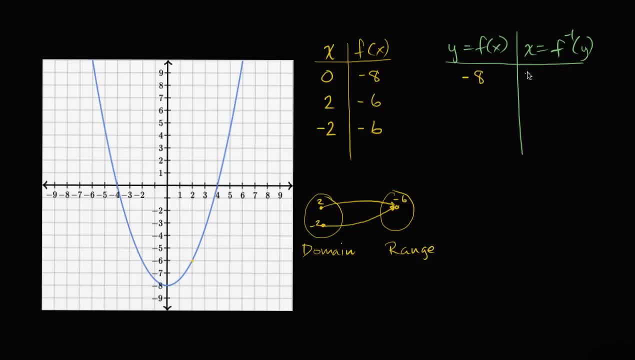 But then we start seeing something interesting, Because the inverse has to be, has to be a function in its own right. And if we say: well, ok, what should f inverse of negative 6 be? And you say: well, gee, there's two ways to get to negative 6 for the function. 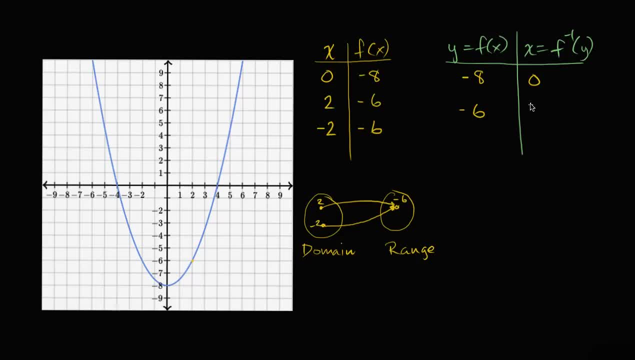 it would go from two or negative two, So the F inverse. if you're trying to do it, you say maybe it's two or it's negative two. Well then F inverse wouldn't be a function if one input maps to multiple outputs. 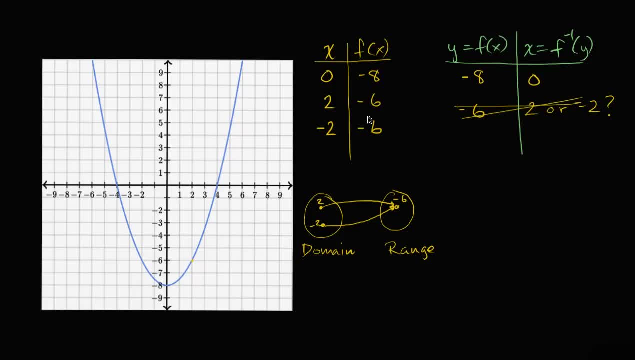 So this isn't okay. So when you see something like this, when you have a function where you have two of its inputs mapping to the same output, you no longer have an invertible function. So this one, as it's defined right over here. 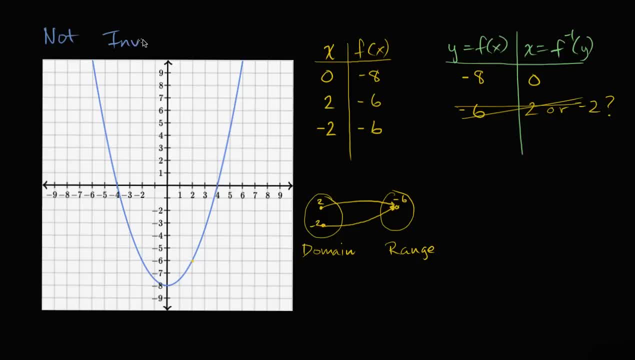 is not invertible. not, it is not invertible. And why isn't it invertible? Because you have two different values mapping to the same F of X, Or actually you have that happening multiple times: Two and negative two. both map to six. 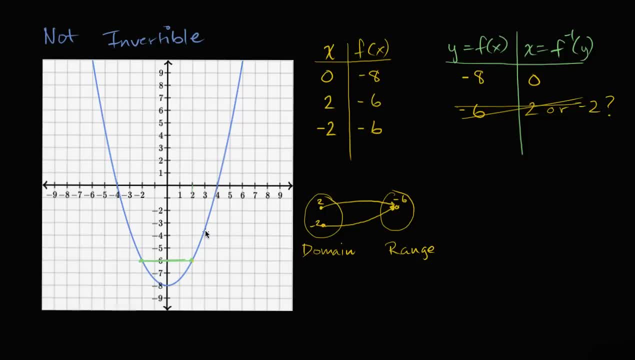 They both map to six Three and negative three. both map to the same value. In fact, this keeps happening. Oh, Over and, over and over again, And so you can start to see. well, maybe there's a test for whether something is invertible. 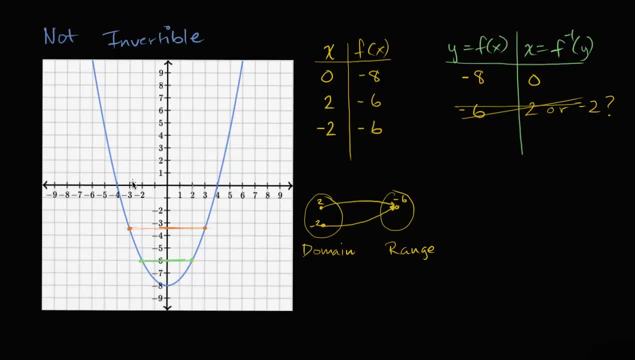 And just as we had the vertical line test for a to see if something can be a function, we could do a horizontal line test to see if it is invertible. And this one clearly fails that, Because with the horizontal line you can see that multiple X values. 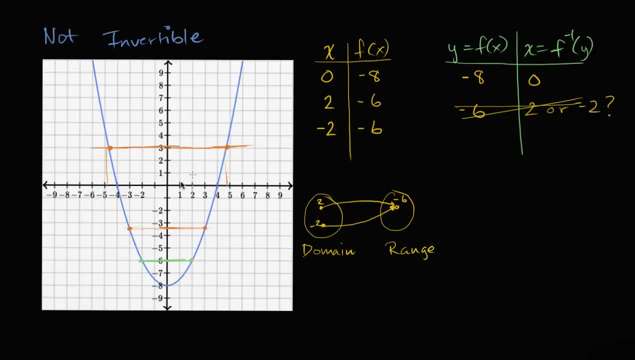 multiple X values can map to the same F of X value to the same. if we say that this is the graph of, if you say this is the graph of, Y is equal to F of X, they're mapping to the same Y value. 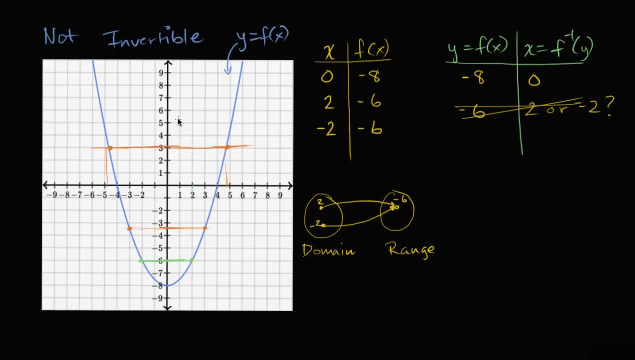 And if they're mapped to the same Y value, then when you try to invert it, that Y value will map to two different X values, And so then the inverse, or this thing that you're trying to construct as inverse, would no longer be a function. 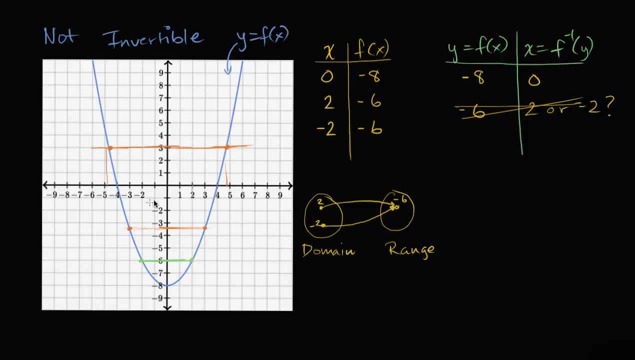 So this thing isn't invertible. But then that gives us a question: Can we restrict? can we restrict this function in some way? Can we restrict the domain of this function in some way so that it could be invertible? And one other way to think about it. 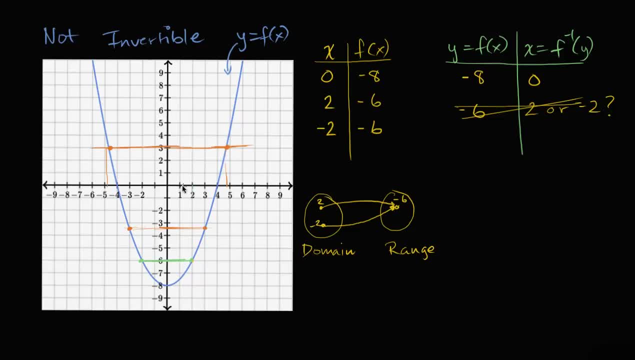 can we restrict this function in a way, in some way, so it passes this horizontal line test? Well, one way that we could restrict this function, one way that we could restrict this function, is if we restricted it only to the right two quadrants. 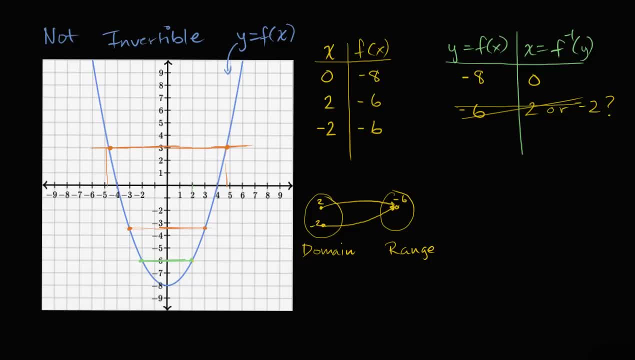 or only to the left two quadrants. So, for example, if you restricted this function to, let's say, the domain going from zero to, actually, you could go to infinity. you could go to infinity if you like. then all of a sudden,